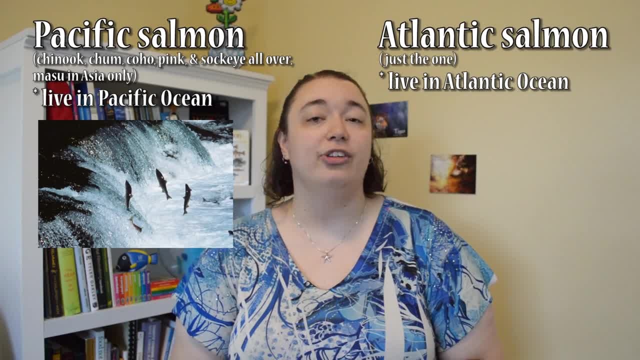 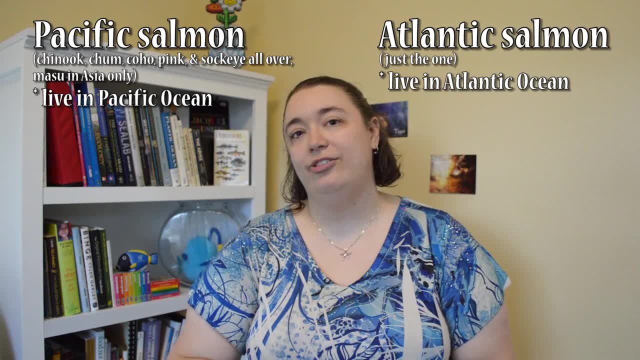 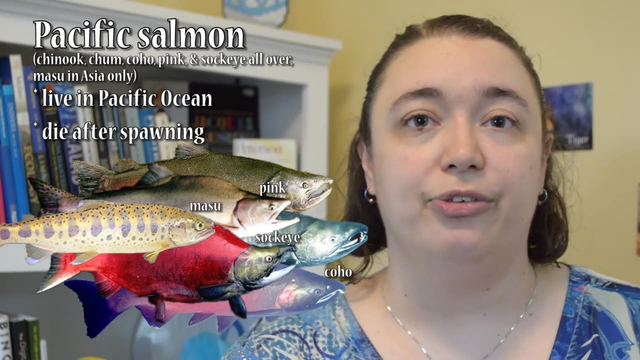 way up rapids and waterfalls to get back to where they hatched, to lay their own eggs, And, of course, they die afterwards. right, That actually only applies to the species in the Pacific. These seven species pour everything they have into fighting their way back to their natal stream to lay or 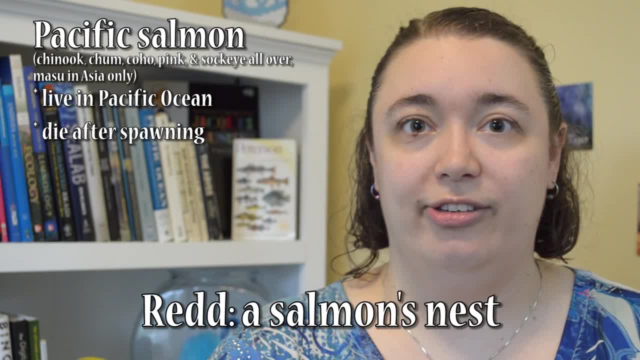 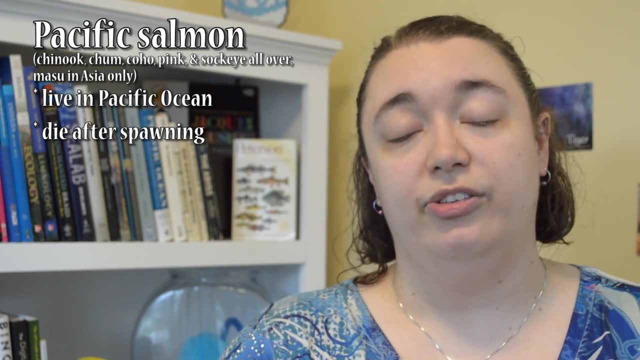 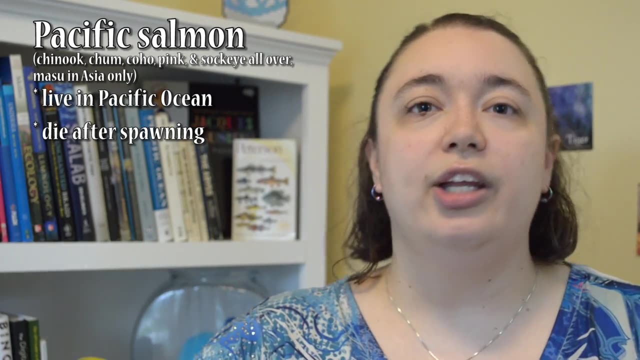 fertilize as many eggs as possible in nests called reds. This breeding behavior is actually similar to a lot of insects, in that once the process gets started, in this case by heading for fresh water, they stop eating and all energy is directed towards getting home and making babies. Shortly after that happens, they 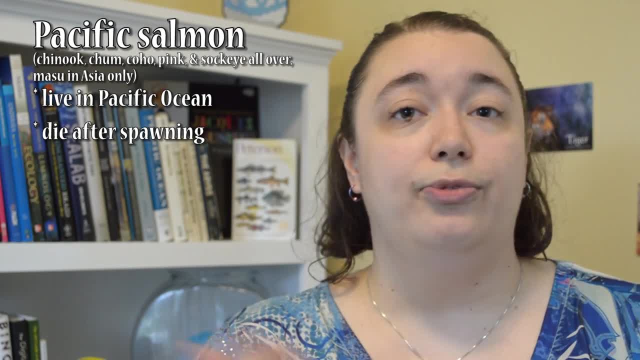 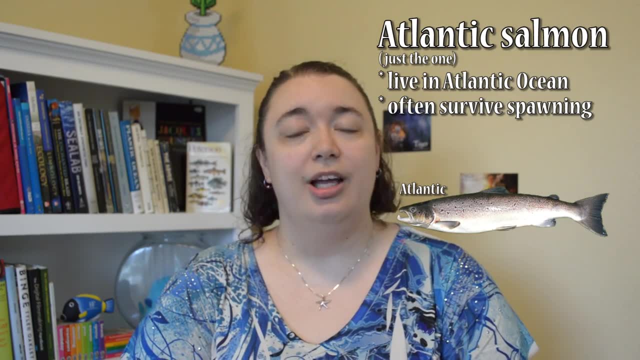 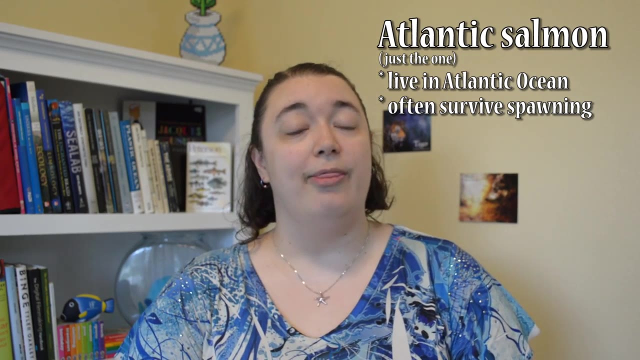 waste away and die, and then they become either fish or fish Food for other animals or nutrients in the ecosystem. Atlantic salmon, on the other hand, often survive spawning. Not much is known about the migration habits of kelts, which are salmon that have already spawned, but we do know that many 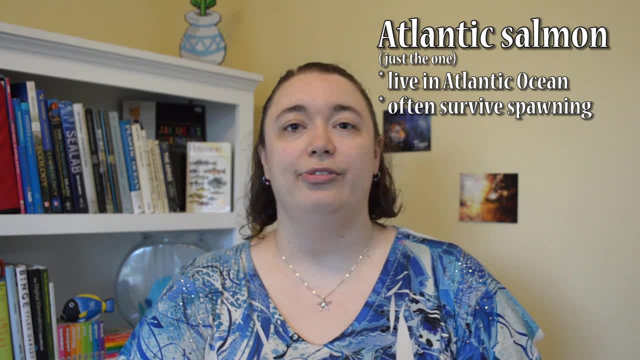 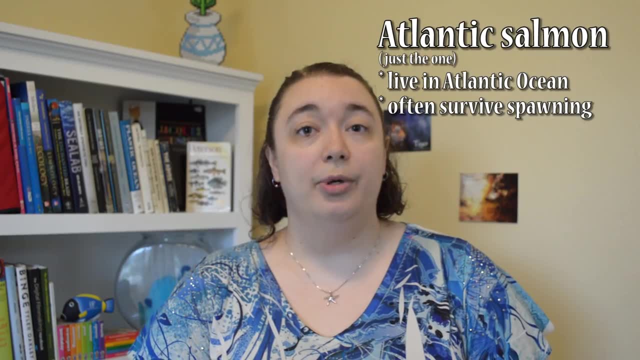 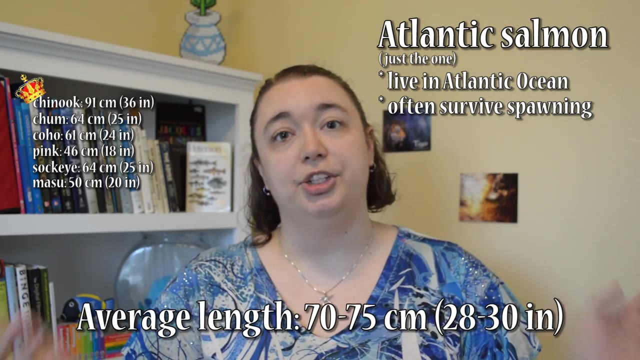 of them make it back to the ocean to rebuild their energy reserves. So why can Atlantic salmon survive the migration when none of the Pacific species can? One possibility is that Atlantic salmon are one of the largest species of salmon, and more bulk means more stored energy. They also don't cut off their own survival systems. the way their Pacific cousins do, so they don't spend the entire migration aging rapidly. They still don't eat once they reach fresh water, and they do seem to need some time to recover before heading back downriver, but many of them eventually do to do it all. 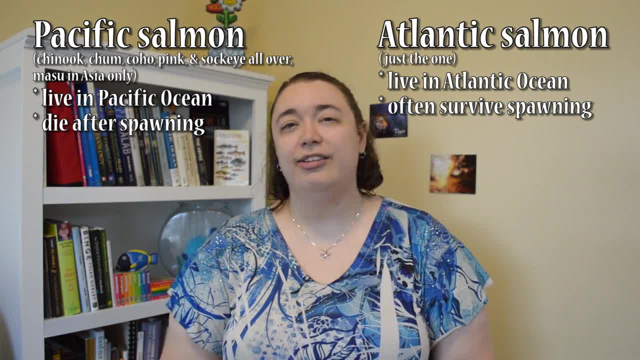 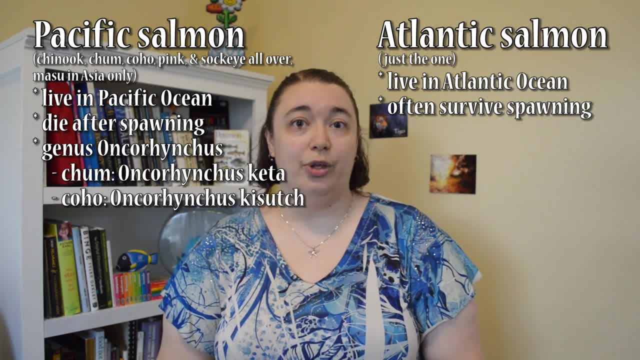 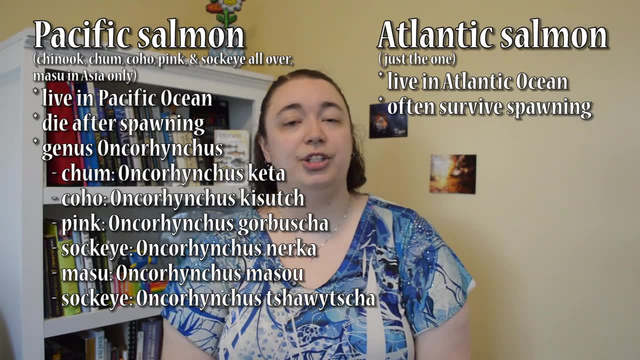 They're not the same genus. They're not the same genus. They're not the same genus. The Atlantic species share genus Oncorhynchus with rainbow steelhead cutthroat trout and other similar trout of the Pacific basin. Atlantic salmon share genus Salmo with brown. 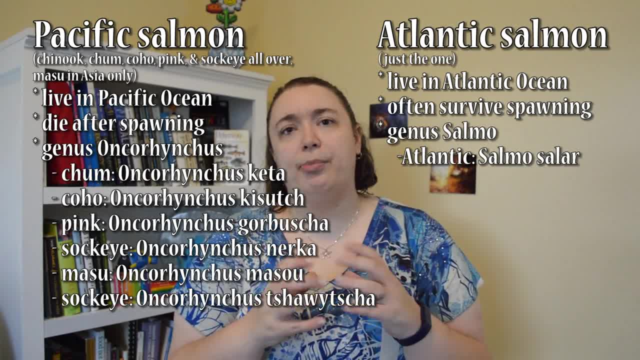 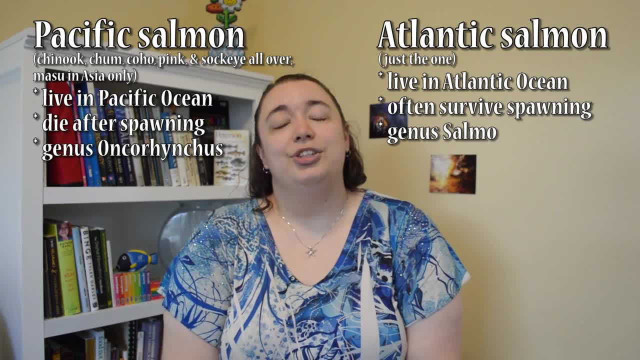 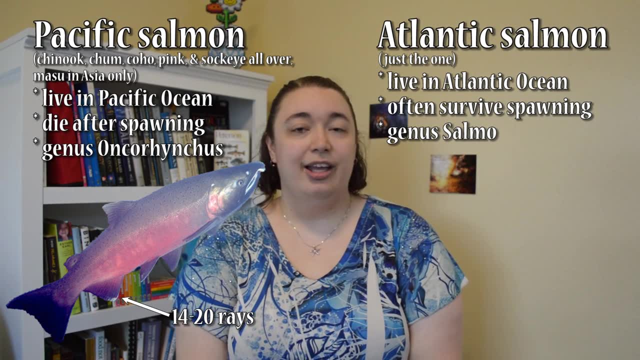 trout and other smaller single watershed populations of similar species. So what's the difference? What sets these two apart? Members of genus Oncorhynchus have 14 to 20 rays in the anal fin, And members of Salmo only have 9 to 12..